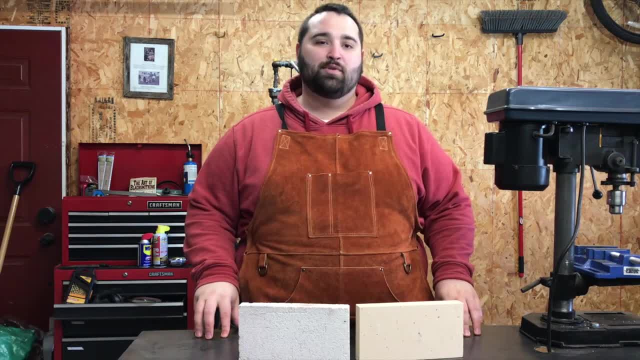 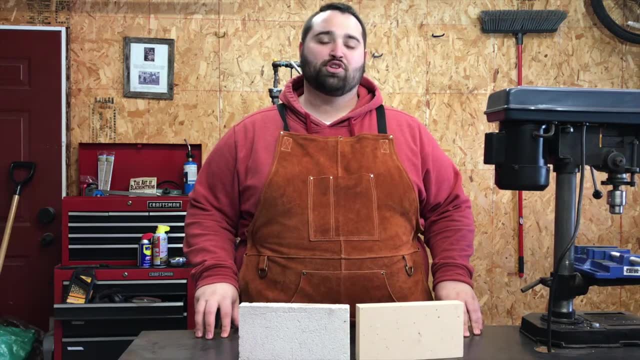 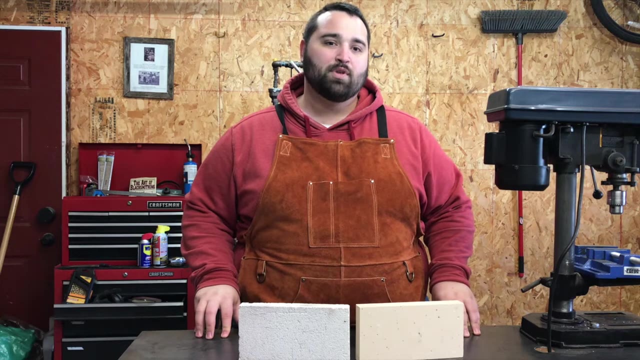 The biggest reason why you shouldn't be using the hard brick in the forge is because they're only rated for the 1800 degrees. When you are going through the forging process alone, forging temperatures start at between 17 and 1800 degrees with a 2% carbon level inside your metal. So 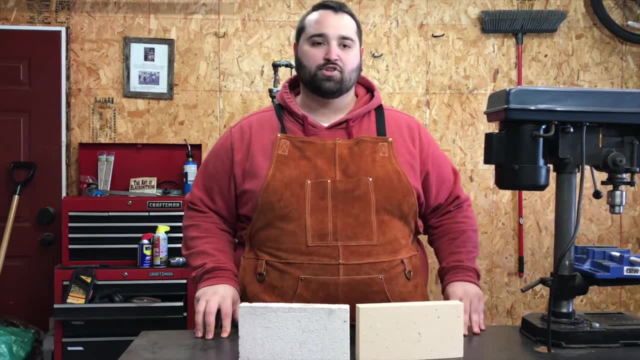 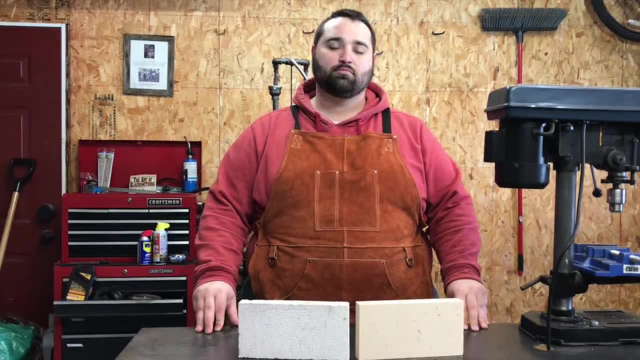 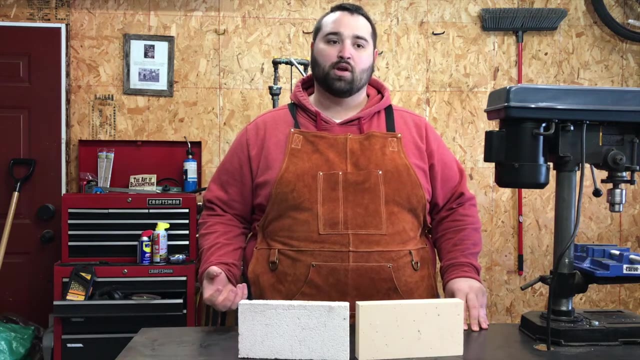 if you're starting off with a hard brick that's only rated for the 1800 degrees, by the time you get to forging heat, you're actually going to melt the bricks out of your forge. Something else to know about the hard brick is they're actually made to pull heat away from the heat source. So 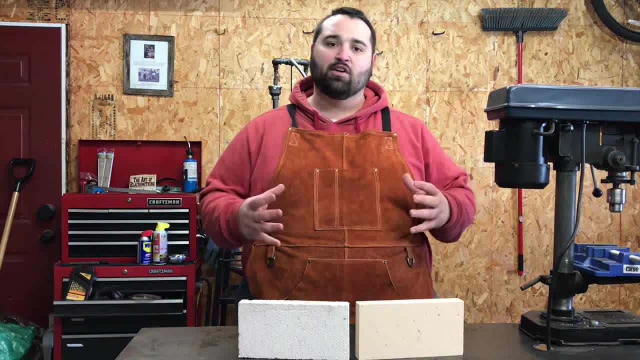 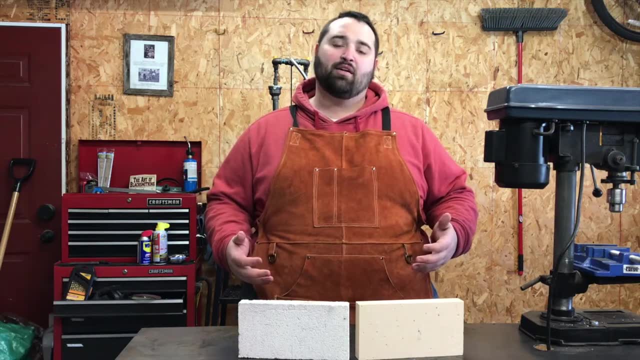 when you're trying to contain all the heat inside your forge and have that heat go into your metal. it's going to take you a lot more time- one- to get to a temperature that you want to. plus, you're going to spend a lot more money in propane costs. 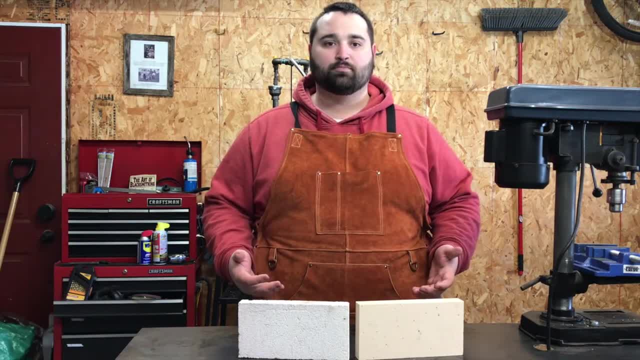 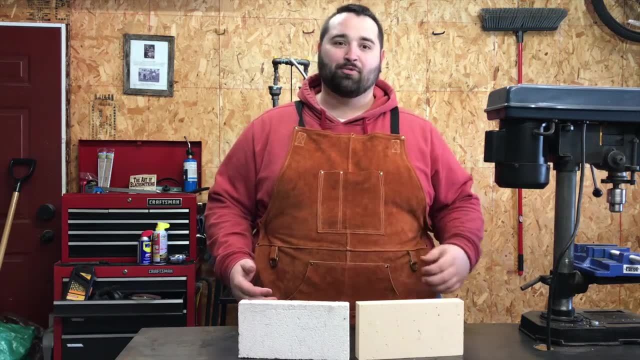 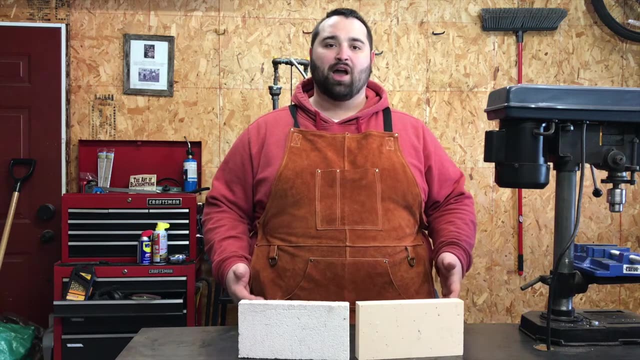 because it's going to take so much to actually heat up your forge. Another common indicator that it's a hard brick is usually they're very hard to work with. If you try to cut them or try to file them to the correct shape or size, it usually takes a lot more effort. 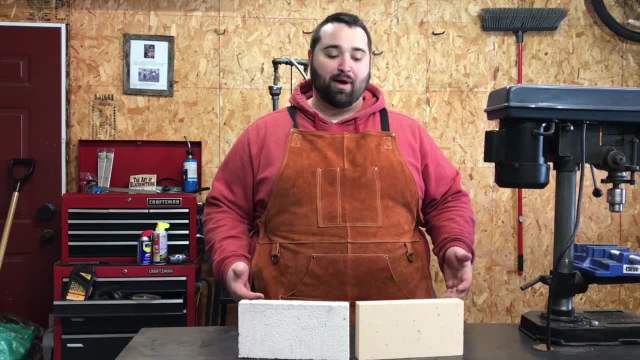 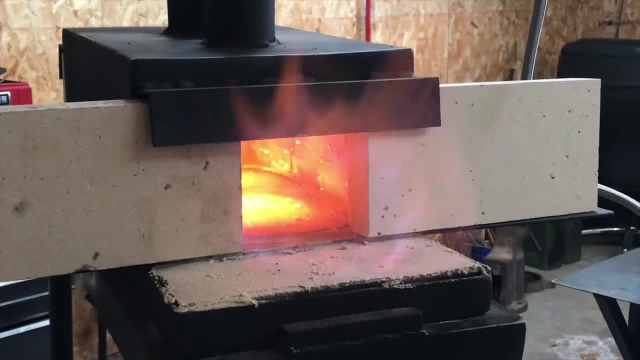 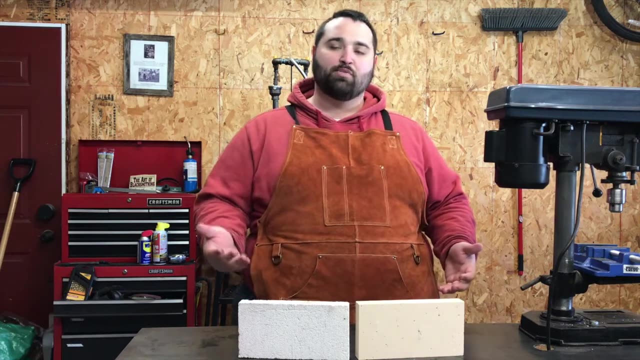 to cut through one of these hard bricks Now in my forge. I like using the hard brick only on the outside. I usually like to use them for making doors to keep the heat in, or if I'm going to do any type of forging with flux, I'll usually put a hard brick in the bottom. 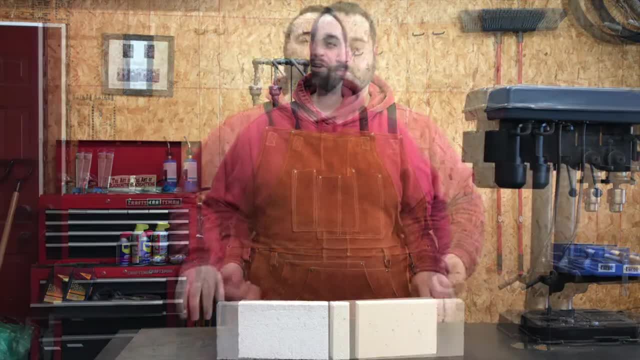 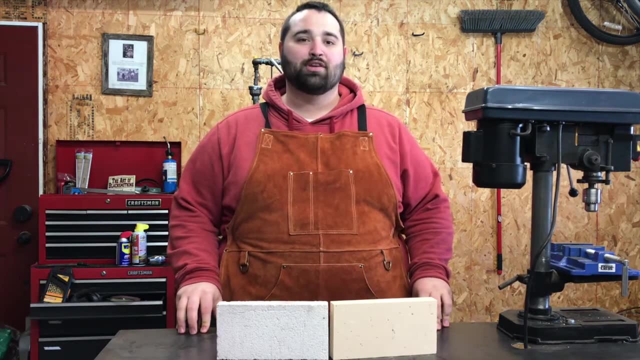 just so I'm not eating away at the bottom of my forge. All right, Now let's talk a about the insulated brick. The insulated brick is also known as a soft brick and typically can't be found in retail stores. You usually have to look online and can find some pretty large 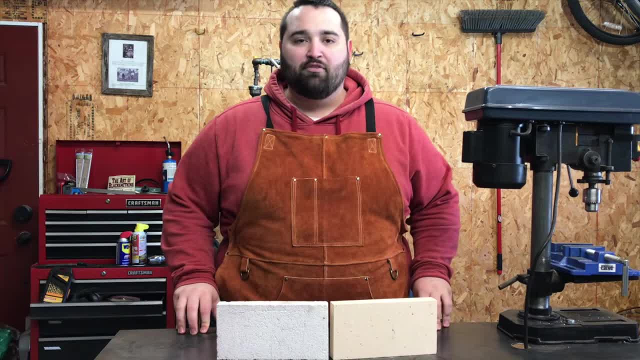 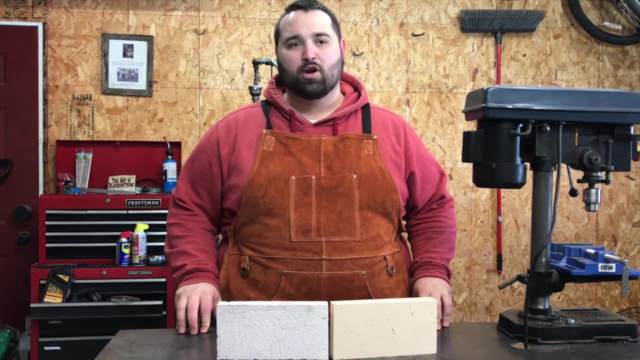 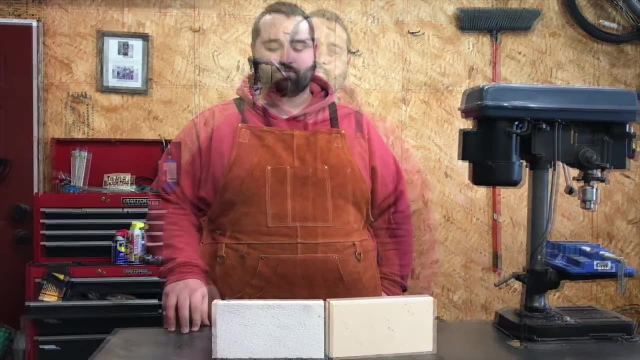 manufacturers that have them. When starting off with a soft brick, you want to use a temperature rating about 2,800 degrees or higher. That way, you will have more consistency in the heat that it's going to hold and will use less fuel in your forging process. When looking at the price point, 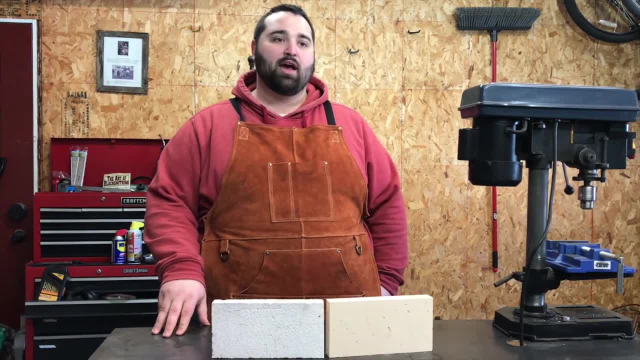 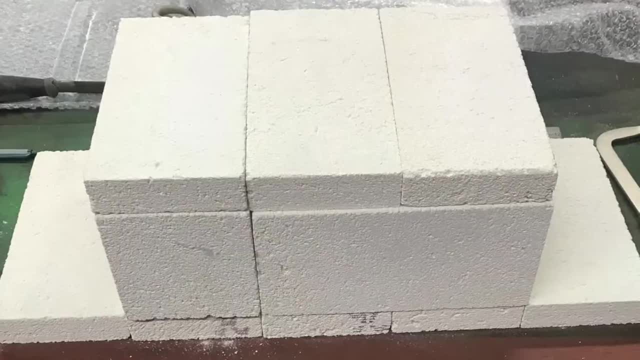 of a soft brick. you're going to want to look at the price point of a soft brick Usually start off at $14 to $15.. I recommend laying out the blueprint of your forge first and figuring out how many bricks you need. The more bricks you can get in bulk typically.